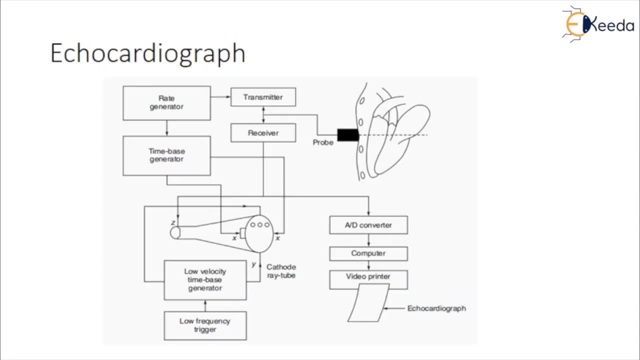 valve, Very important use in the detection of pericardial diffusion, which is the abnormal collection of the fluid between the heart and the pericardial sac. The examination can be performed quickly and easily at the bedside without apparent risk to the patient. 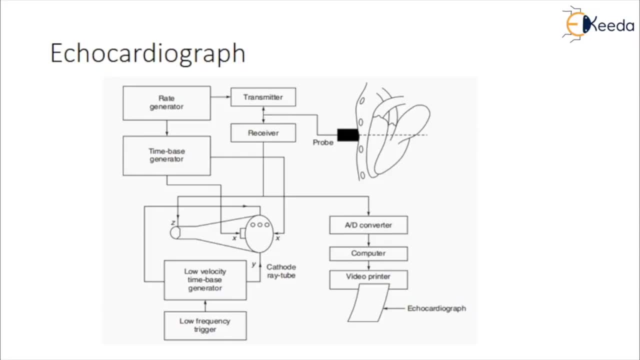 Ultrasonic echos produce vertical displacement of a horizontal trace on CRP. The amount of vertical displacement is proportional to the strength of the echo, and the distance along the horizontal trace represent the time of the sound travel in human tissue, thereby permitting accurate measurement of tissue depth between any two echo sources. A digital echocardiography. 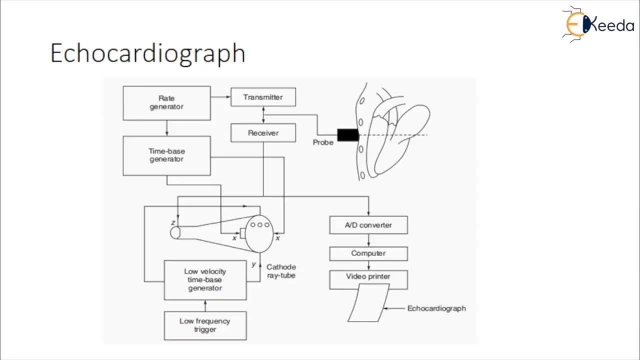 which involves recording, displaying and storing an echocardiogram digitally, has therefore largely replaced the videotape recording procedure. Measurement and interpretation can be done more conveniently using digital techniques of recording and manipulating imaging information For electrocardiography. the transducer is placed between the third and fourth ribs of the outer. 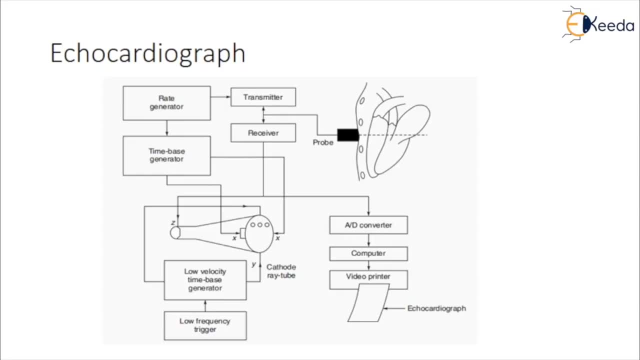 chest valve, where there is no lung between the skin and heart. From this probe, a low-intensity ultrasonic beam is directed towards the heart area and echo signals are obtained. The probe position is manipulated to obtain echoes from areas of interest in the heart. 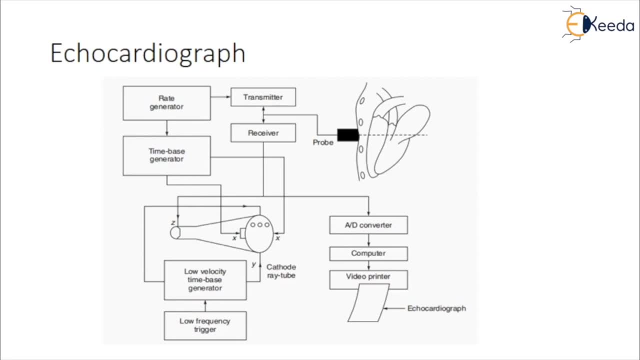 A growing number of routine examinations and the possibility of extracting more quantitative data from the echocardiogram has necessitated the development of computer systems for semi-automated analysis of M-mode echocardiogram. The routine program generally aims: the measurement can be subdivided into three groups. 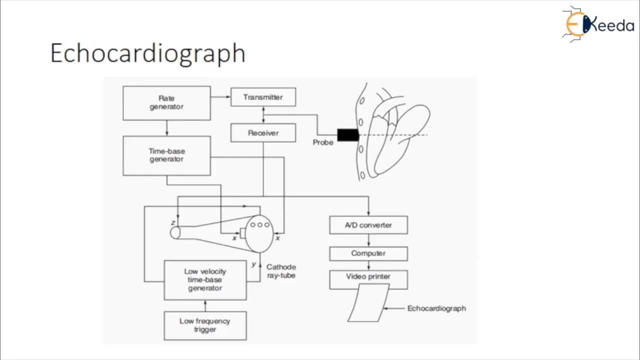 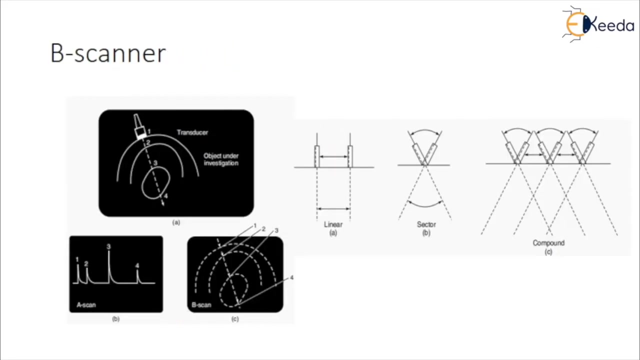 dimensions. ultra and left atrium dimensions. mitral valve measurement. Each group of the measurement is preceded by a calibration so that it is possible to use different recordings for the measurement of structure from each group. Here it is a B-scanner diagram. It is shown. 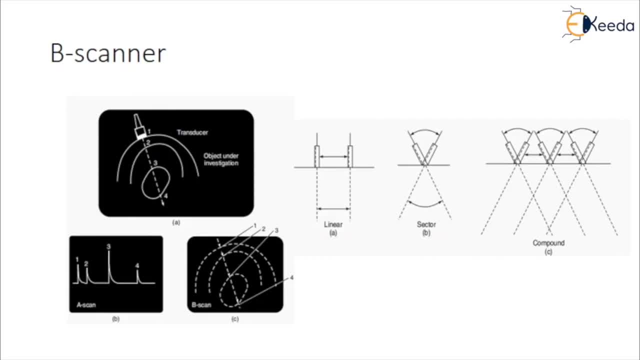 B-scan is based on the fundamental information provided by ECOS in an A-scan mode, which is used to modulate intensity of the CRT electron beam instead of deflecting it vertically. for obtaining two-dimensional cross-sectional image B-scan, It is necessary to know the transducer position. 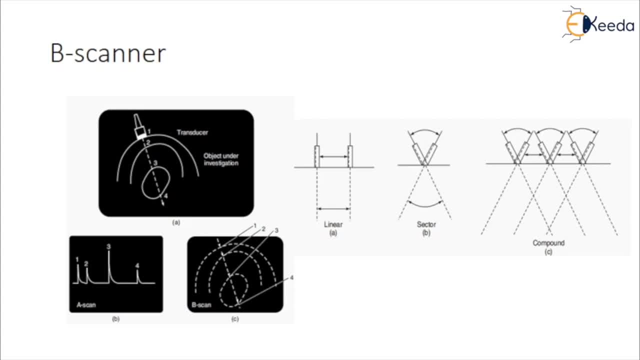 and its orientation. The transducer is moved manually for scanning the region of the interest area. and a transducer is coupled by shaft encoder and position sensor to the coordinate generator so as to correlate the origin of the ECOS from various structure of the body on the CRT screen. 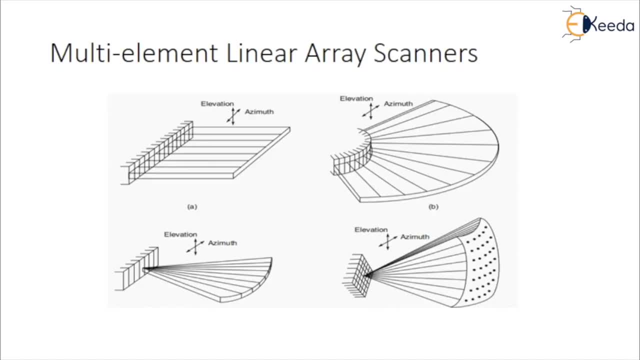 Multi-Element Linear Array Scanners. Array transducers are available in several element configuration. Their arrangement determines the shape of the scan. for dimensional image, The scanning plane is the same dimensions, whereas the elevation dimension is perpendicular to the assumed scanning plane. The shape of the region scan for various array element. 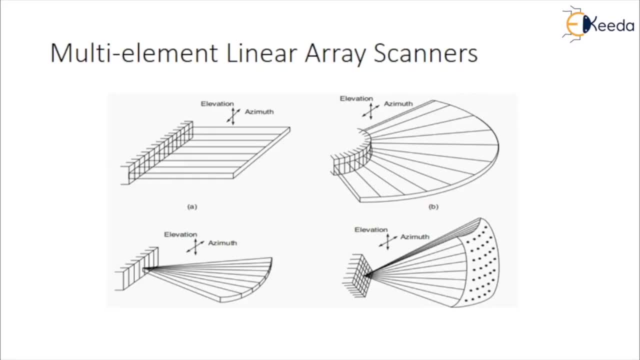 configuration: Linear Sequential Arrays. The sequential linear array scans a rectangular path. The scanning lines are directed perpendicular to the face of the transducer. The beam is focused but not steered. Linear array transducers are available with 512 elements in currently available ultrasound scanners. 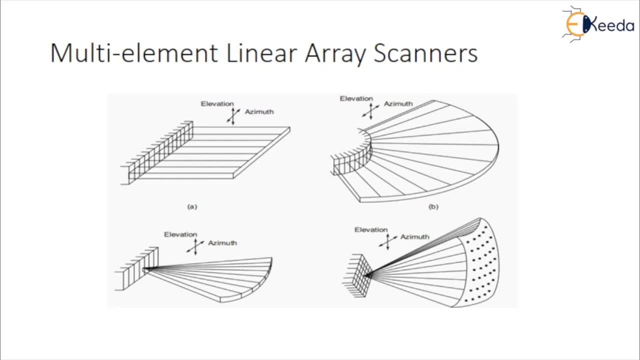 Curvy Linear Arrays. A curvy linear array scans a wider field of view because of the convex arrangement of the array elements. Curvy linear or covax convex arrays operate in the same manner as the linear array. Curvy Linear Arrays are capable of scanning the events of the curve in order to obtain 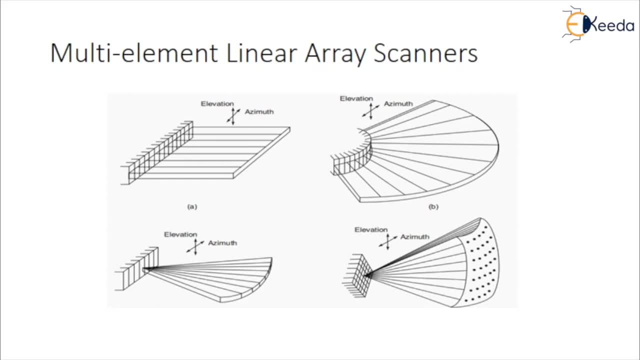 the current appearance, They can be used for scanning the individual elements of the trace finger arrays. therefore, even in this case, scan lines are directed perpendicular to the transducer phase Linear phased array which is shown in the third figure. the arrangement of the elements is similar. 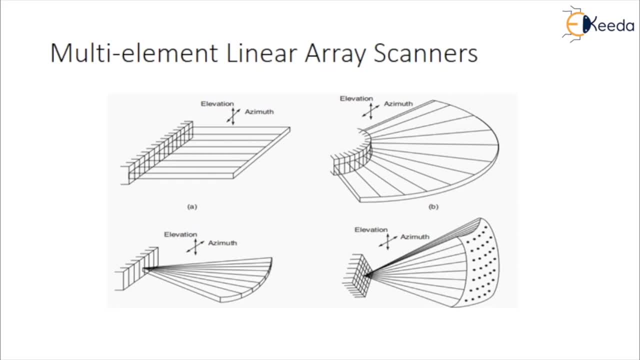 to the linear sequential arrays, but the scanner steers the ultrasound beam through a sector shaped region in the azim plane. The present linear phased arrays is up to 128 elements and all the elements are used to transmit and receive each line of the data phase. 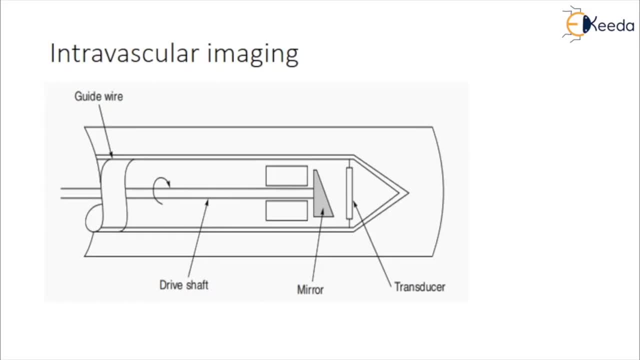 The device comprises a fixed transducer element at the tip of the catheter and rotating mirror driven by an external motor. A flexible drift shaft. by using this device, we can obtain radial cross sectional images of the artery. After placing a guide wire in the coronary artery, the catheter is passed by guide wire control. 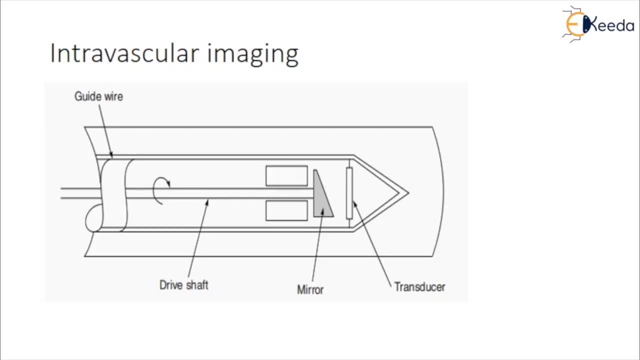 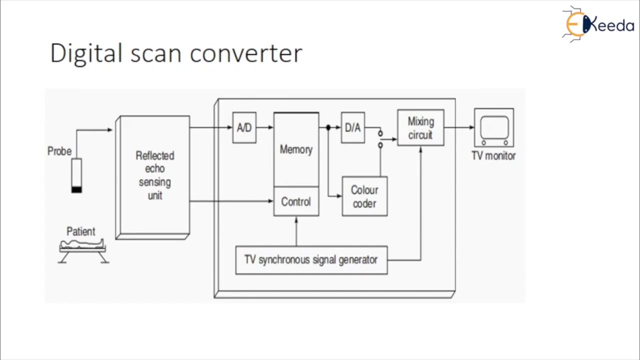 into the selected area of the artery and positioned under fluoroscopic control. The outer diameter of the catheter is typically 1.4 mm. At an ultrasound frequency of 30 megahertz, high resolution images of the vascular pathology are obtained. Digital scan converter. Lines of ultrasonic information are not generated in TV compatible. 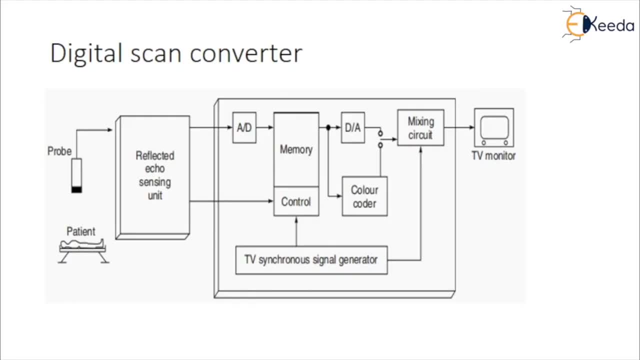 format. Consequently, to use TV monitors to display the image, some kind of scans conversion must be performed. The majority of scanners digitize the image information, use digital memory as a buffer store. The memory can be updated. they are never required. and to use a standard video output, Digitization of the echo information can be performed. 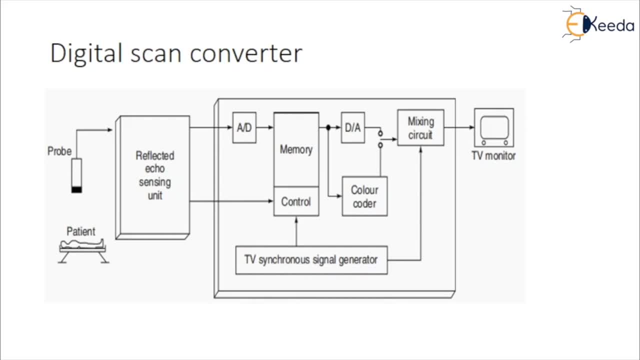 at a number of points in the signal processing chain. The most convenient is just after demodulation and video processing. The dynamic range is about 50 dB and the required digitization rate about 1 megahertz. This criteria is readily available. analog to digital converter. Digital scan converters used in commercially available scanners. 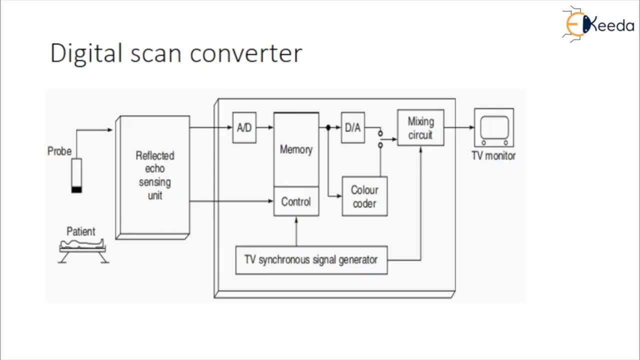 provide storage arrays with picture elements 512 x 512.. The scan converter control receives signals of transducer position, ultrasound velocity control and TV synchronization pulses. Generates X and Y addresses Information which is fed to the digital memory. The echo signal is given to an analog to digital converter. The digitized information goes to the memory after. 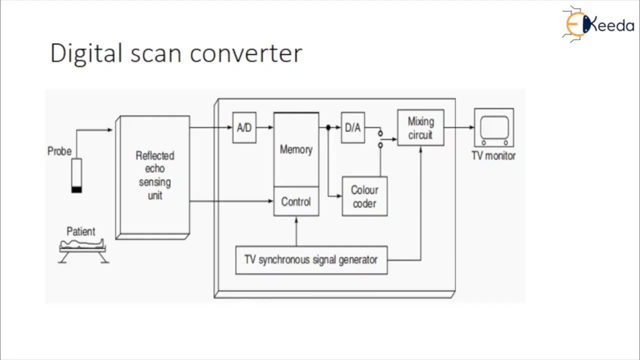 input, holding register and read write logic. Digital scan converters are microprocessor based and offer several additional benefits to the user. Alpha neural information concerning the patient, date and equipment. parameters such as transducer, frequency, scan settings and locations of the scan plane can be conveniently entered. 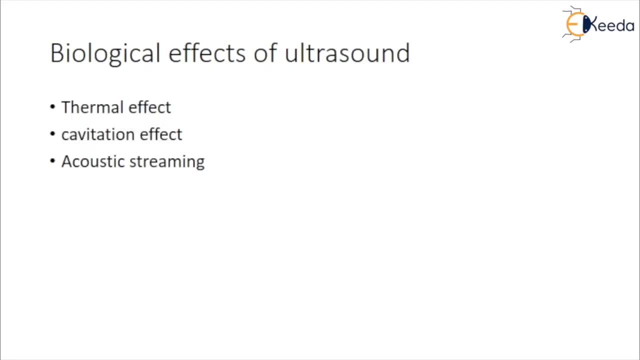 and displayed along with the ultrasound image. Biological effects of ultrasound. Ultrasonic radiation in clinical use is known to be substantially less hazardous to tissues than radiation like x-rays, which are in common use in some of the same applications. Significant attention has been given to the investigating the effects of ultrasound on biological tissues. 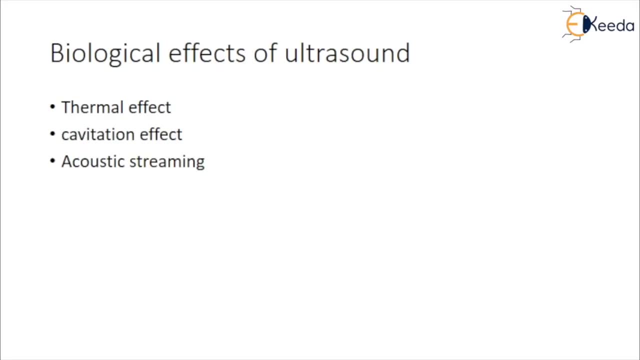 It has been reported that ultrasound affects biological tissues via three main effects: Thermal effect, cavitation effect and acoustic streaming. Thermal effect: a tissue has high protein content, A high intensity of a continuous wave ultrasound is used, Bone is included in the heated volume and vascularization is poor. 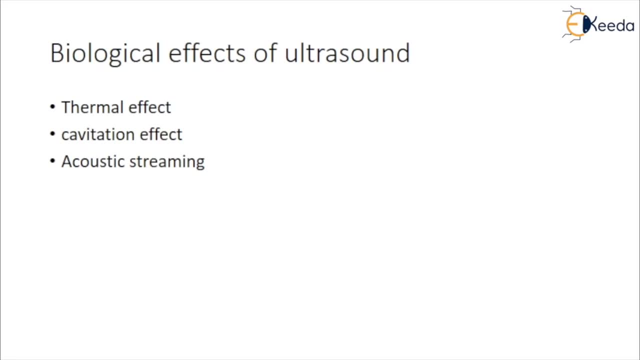 Cavitation effect may be important when low frequency ultrasound is used. Grassy fluids are exposed. Small gas is the main source of the ultrasound and playing generator. as filled spaces are exposed, the tissue temperature is higher than normal. Acoustic streaming may be important When the medium has an acoustic impedance different. 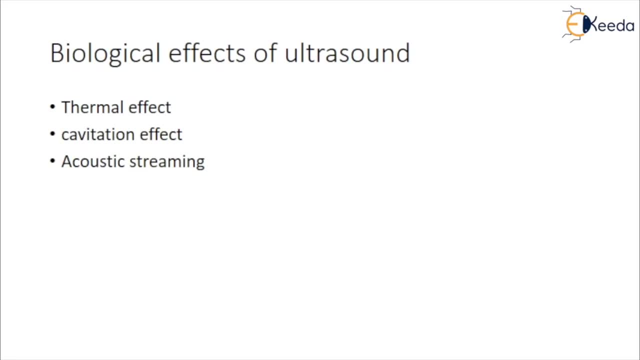 from its surrounding. the fluid in the biological medium is free to move. more continuous wave application is used. Mechanism of Cavitation: Cavitation occurs due to the nucleation of small gaseous cavities during the negative pressure cycles of ultrasound, The cavitation leads to the disordering of lipid bilayers and formation of aqueous channels. 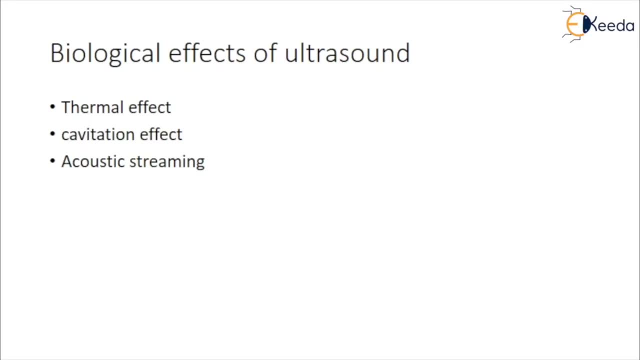 in the skin through which drugs can penetrate. Cavitation inside the skin cavitation bubbles near the keratin sites, lipid bilayers interfaces- in turn cause oscillations in the lipid bilayers, thereby causing structural disorders. Cavitation bubbles can potentially play a role in the observed transdermal transport. 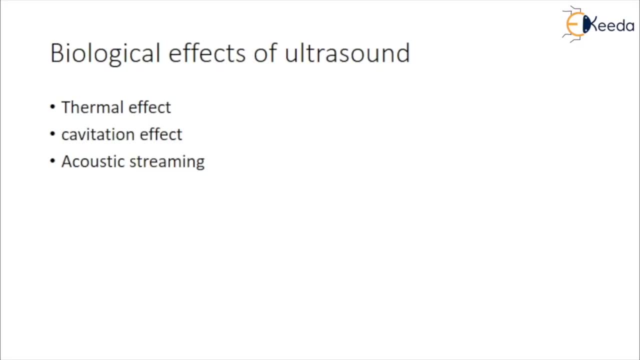 enhancement. These bubbles cause skin erosion due to generation of shock waves, thereby enhancing transdermal transport Thermal effect. Absorption of ultrasound results in a temperature increase of the medium. Materials with high ultrasound absorption coefficients, such as bones, experience several thermal effects compared to the muscle. 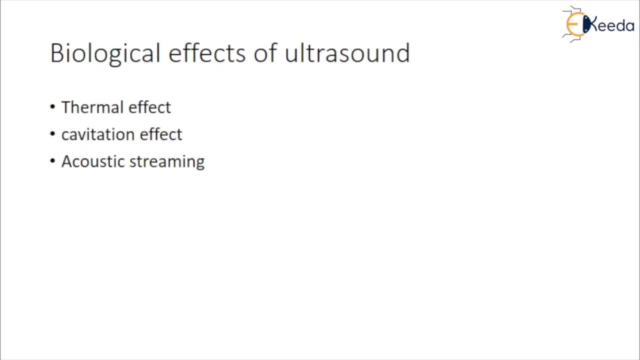 The body is also exposed to the heat of the body. The body is also exposed to the heat of the muscle tissues which have a low absorption coefficient. Absorption coefficient of a medium increases proportionally with the ultrasound, indicating that thermal effects of ultrasound are proportional to the ultrasound frequency. The increase in the temperature of a medium.